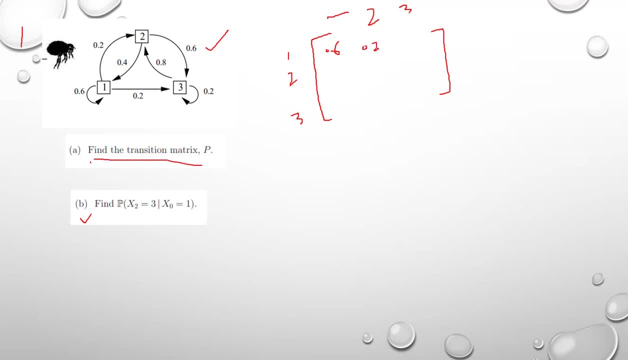 0.2, 1, 2, 2 is 0.2, then 1 2, 3 is also point point. okay, now we can go to the class 2, 2, 2, 1 is 0.4, 2, 2, 1 is 0.4 2, 2, 2 is 2, 2, 2 is 0. 2, 2, 3 is 0.6. 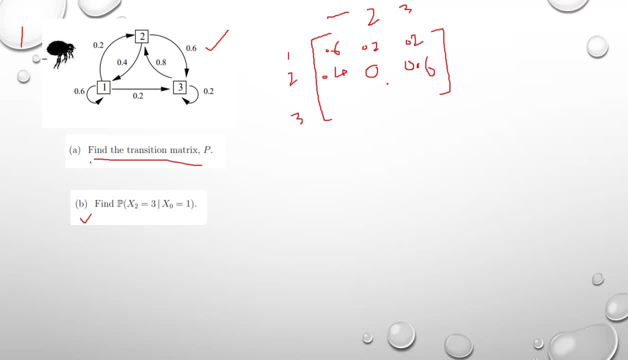 2 2 2 is 0.6. okay, then go to the 3: 3 2 1 is 3 2 1 is 0. 3 2: 1 is 0. then 3 2 2 is 0.8. 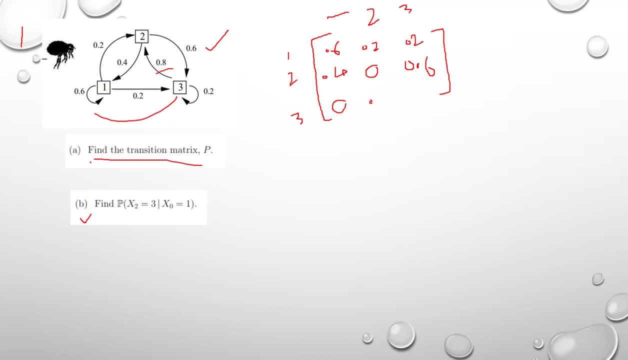 3 2 2 is 0.8, 3 2 2 is 0.8 and 3 2 3 is 0.2, 3 2 3 is 0.2. when you add up all rows, you got one one, one columns also 1, so this thing is. 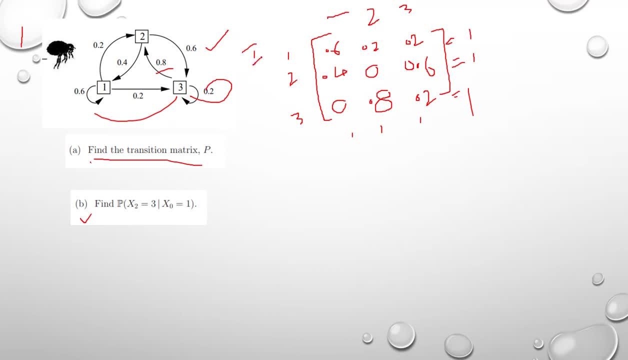 irreducible, then is irreducible. now we need to find this probability value: probability of X 2 equal to 3, given X 1 equal to 1. this is two steps probability, two steps probability. so P square, which value C is P 1: 3. 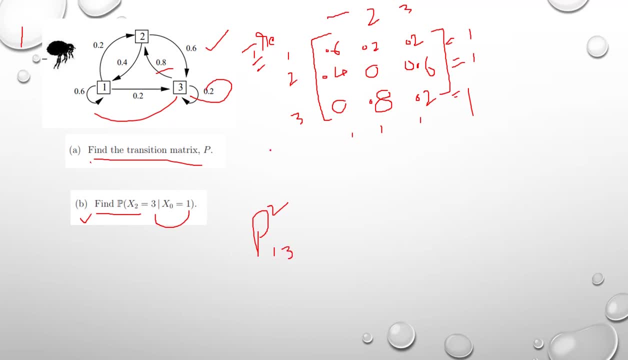 P 1- 3. I am denoting with this matrix 2 P. then I need P square. in P square I need value of P 1- 3. means this, this type of value I need after multiplication, so first we can multiply. so P square 1- 3 means we don't need all, well all. 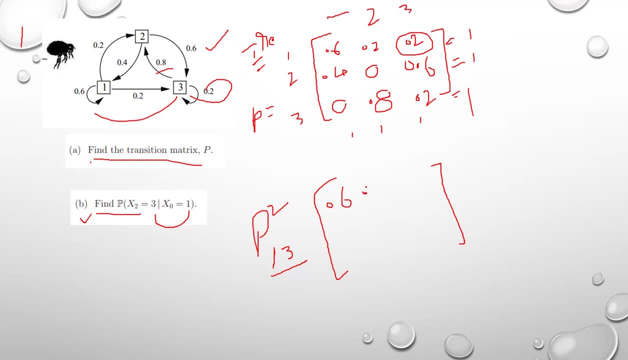 calculations. for time saving, we are taking one row on the broad column on. okay, you can take all that. rose also that after calculating this, you can finally get P 1: 3 value. this is the question number 1. okay, you can finally get P 1: 3 value. this is the question number one. okay, now we yeah, yeah, you can take your values okay. so essentially, this actually is good, Because we can take the answer three times in one row and in two round. column value this way: P 1- 3. after calculating this one row, this will get P 1- 3, or as: 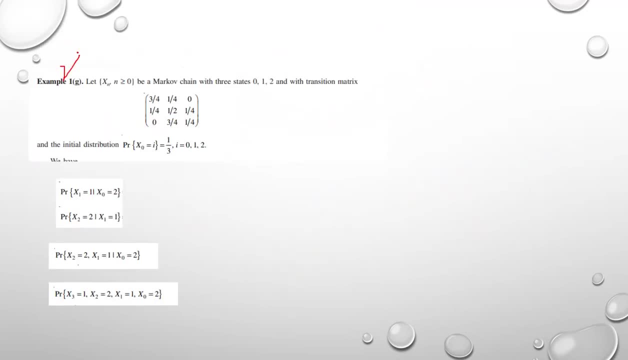 we can go to the second question. this is question number two. okay, let xn and greater than zero be a markov chain with three, three states, zero, one, two and with transition matrix. this is my transition matrix and initial distribution is also given. now i want to find this probability of x1 equal to 1. 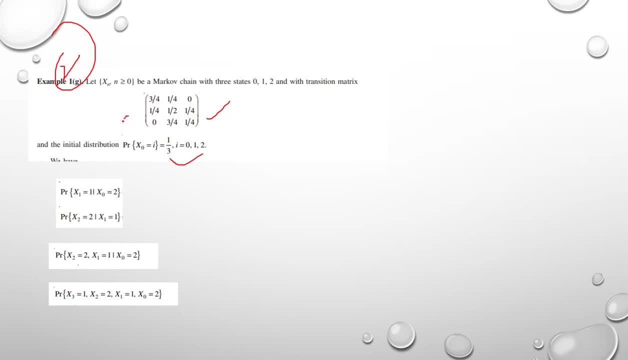 and x naught if this is one step probability, so we can find values from this matrix. so probability of x1 equal to 1, x not equal to 2 is 3 by 4, 3 by 4, 3 by 4. i need probability of 2: 1, probability of. 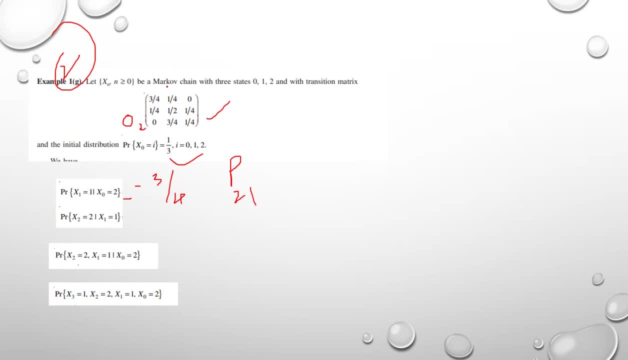 2. 1 is what here? 2, here 1. so i got this value. this is 3 by 4. now i need 1: 2 value. 1: 2. 1 2 value is 1 by 4. 1: 2 value is 1 by 4. 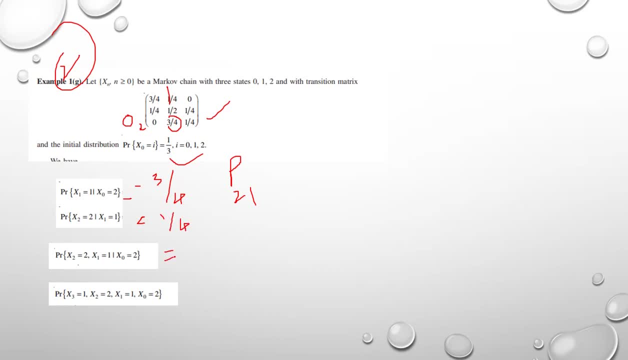 now i need this how we can write. we can write it as: probability of x2 equal to 2, given x1 equal to 1, these two probabilities multiplied by x not equal to 2, then finally we got 3 by 4 and 1 by 4. 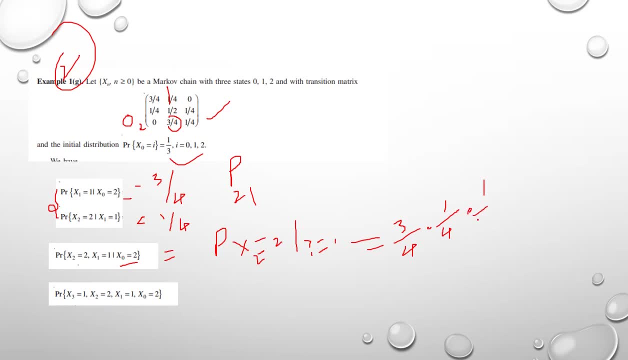 initial probability is 1 by 3. when you can calculate this, you get some value. final answer is 1 by 16. okay, now, if we find this value. for finding this value, formula is: you can calculate it. formula by directly: also we can calculate it. see how we can calculate. 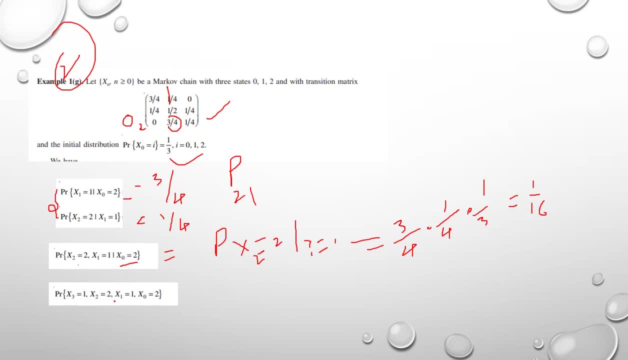 this. we can write it as x3 equal to 1, x2 equal to 2, x1 equal to 1 and x naught equal. so we can write it as probability of x3 equal to 1, given x2 equal to 2, x2 equal to 2, then multiplied by x to one relation and. 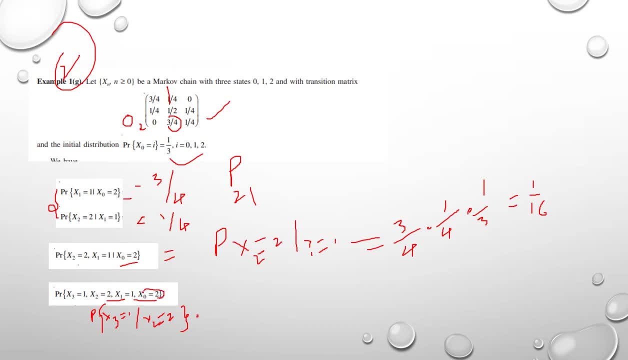 1- 2 relation. finally, X not equal to 2. so finally, what we need: probability of 2- 1 multiplied by probability of 1, 2 multiplied by probability of 2, 1 multiplied by probability of X not equal to 2. here we got 1 by 3 in here. 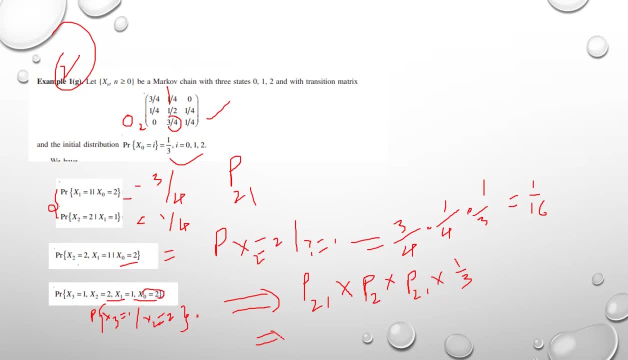 distribution, so you can just substitute values. probability of 2: 1 is 3 by 4, 1, 2 is 1 by 4 and again 3 by 4 and one by 3, 3 by 4 and one by 3. some values are: 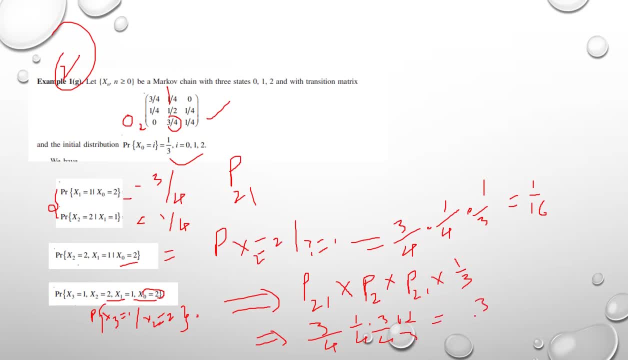 cancelled. finally we got 3 by 4 cube in 64. this is the final answer for this question is simply: we can collect in this person. these are our one-step probabilities. here we have all our one-step probability, so we have moved on. this is important. topic: periodicity. 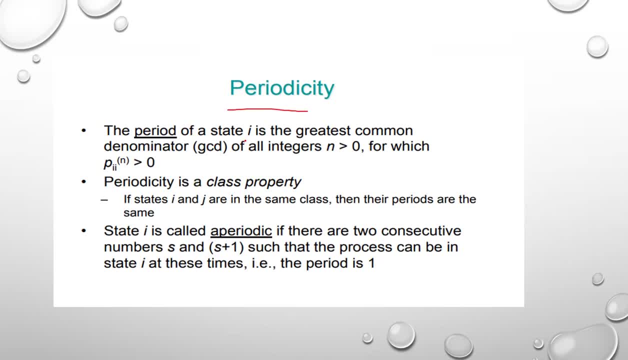 periodicity. the period of a state I is the greatest common denominator of all integers and greater than 0, for which P, I, any current periodicity, is a class of probability. if state I and J are in the same class, then the period are the same. these all are the points to remember when you are doing periodicity problems. 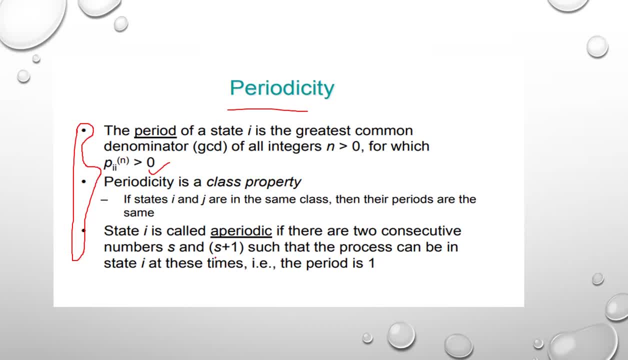 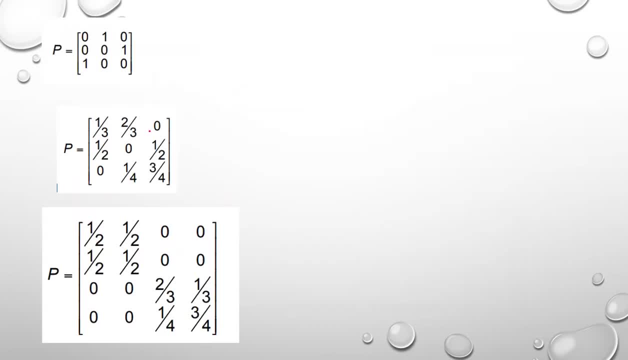 state, I is called a periodic if there are two consecutive numbers- s and s- plus one. such as a process can be also be stated this: now we can see examples, this: examples are important thing. first we can make graph, okay. first we can make graph from here: one, two, three, here also one, two. 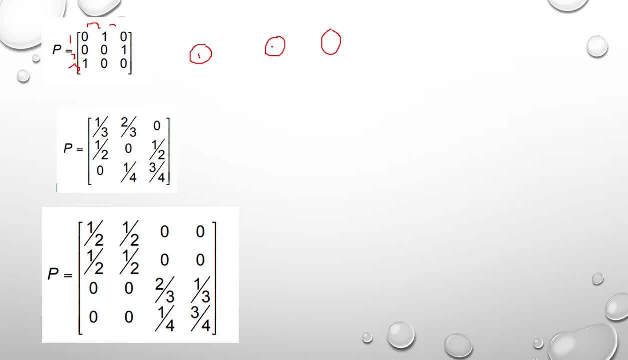 three, one, two, three, one, two, two, one, two, two is one. okay, then two, two, three, two, two, three is one. okay, then three. two. one is one. when you can write G seed of each class, GCD, you write G, C drift for Class one. how many times, how much time take 1, 2, 3, 3. 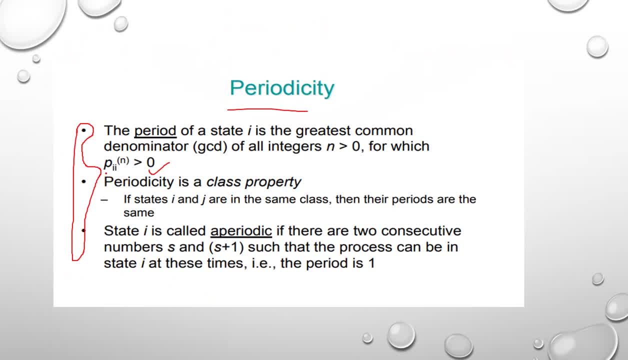 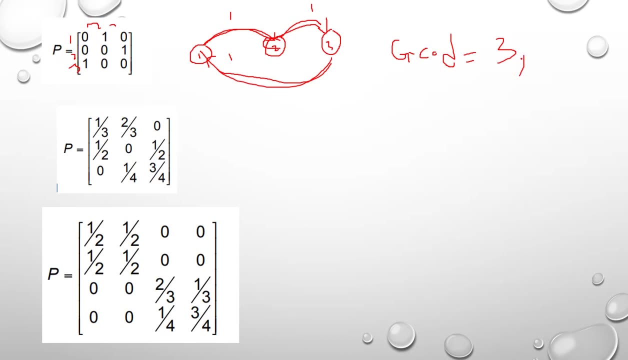 C, observe what is question: probability of a state and high state for enemies. we need same state so you can calculate for tool also, for tools will get three, but was always机 3, 3, ok, ok, 3, but three also we get three. so here get test common device. three is three, so period of this. 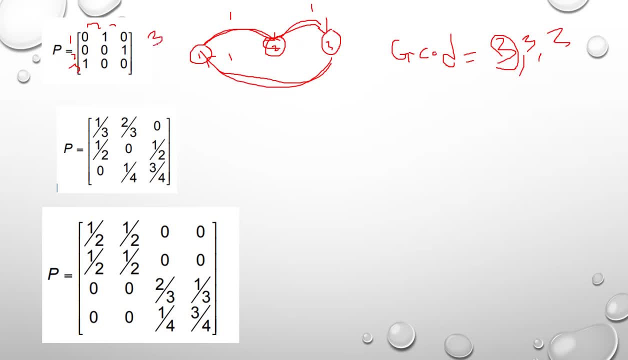 transition matrix is three and chain is irreducible. chain is irreducible. okay, now we can see this. examples also. first we can formulate graph: one, two, three from one to one is one by three. one two, one is one by three and one two, two is two by three. 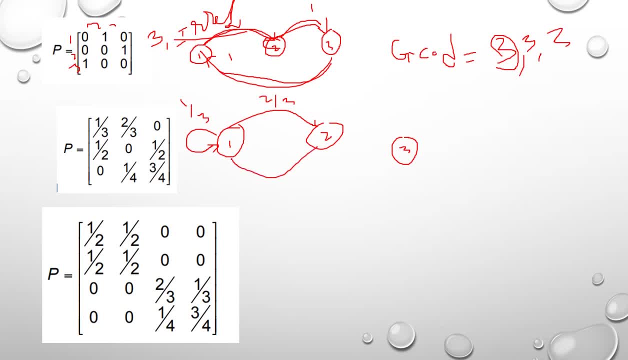 then two, two, one. two, two, one is one by two and two, two, two is zero. two, two, three is one by two. two, two, three is one by two. then three, two, two is one by four. three, two, three is three by four. okay, now we can check for this gcd, this chinese gcd is one by four. 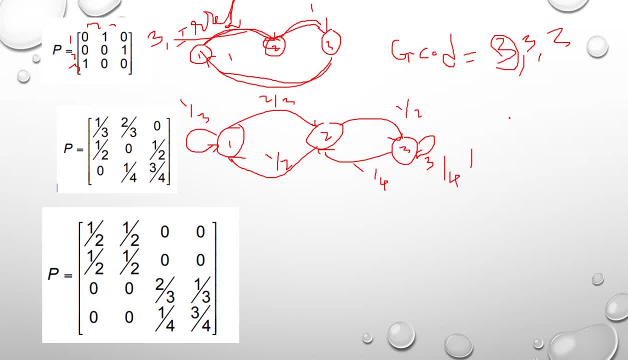 by seeing we are saying that this thing is irreducible. irreducible, this chinese it is. now you can find for periodicity, for finding pictures: if you take class one for class one, it take one in one step also possible. okay, for class two, it take two steps also. for class three, take one step also. if you find gcd, then gcd. 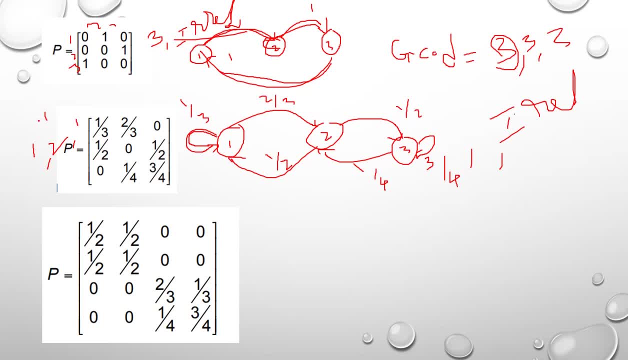 gcd is one. so this is a periodic class, a periodic. yeah, this is three period, three period, a period. now we find for this by observing this: okay, all are greater than zero, then we say that this is a periodic. if diagonal values are greater than zero, then we can say that this is a period. this is one result also. you can see here also. okay. 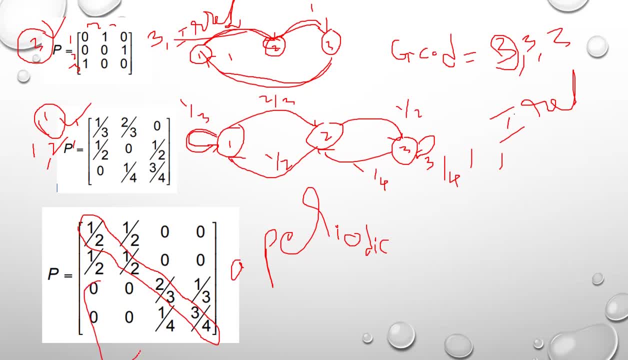 by simply, we are saying that this is also reducible. this is not irreducible. this is a reducible chain. when you can formulate a graph, that time you got reducible and not. this is not irreducible. now we can go to the recurrent state and 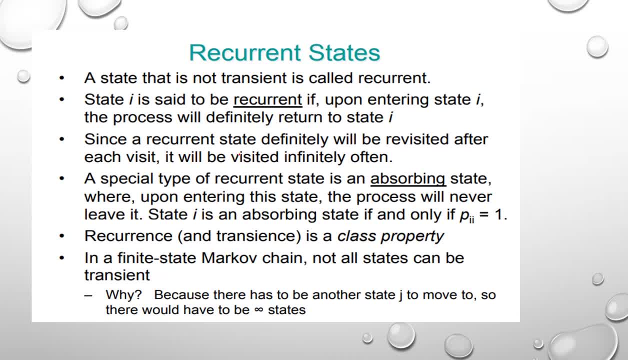 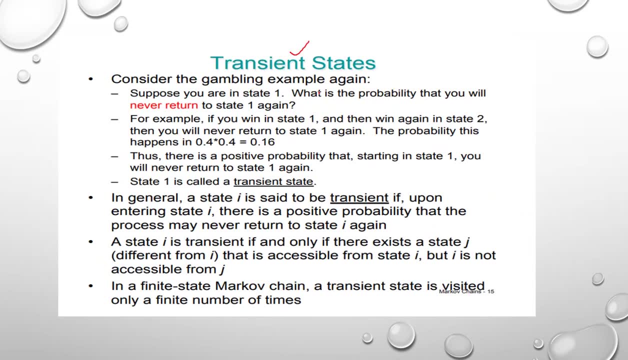 persistent, transient, all things. we can discuss this here. see what is recurrent, what is recurrent. a state that is not transient is called recurrent. before that transient, recurrent- we can see transient, what is transient state. consider the gambling example again. suppose you are in state one, what is the probability that you 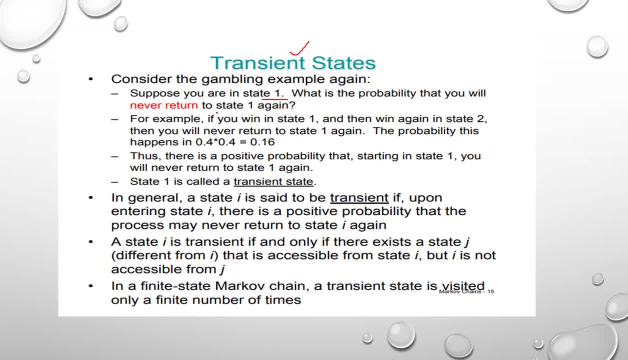 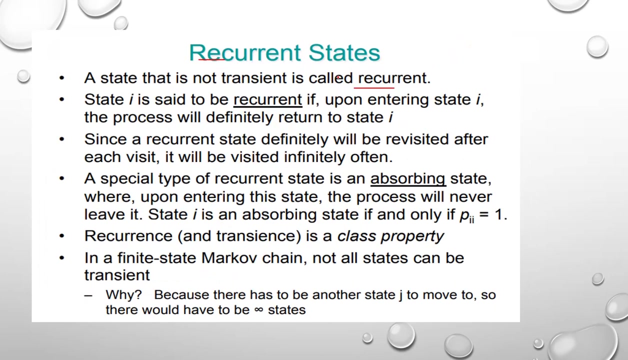 will know, will never return to state one again never means. when you see the examples, that time you can easily understand. but i will now also. i will try to understand how here, when you calculate f, y capital, f is not equal to one, that time we say that transient when equal to one, it is recurrent of persistent. 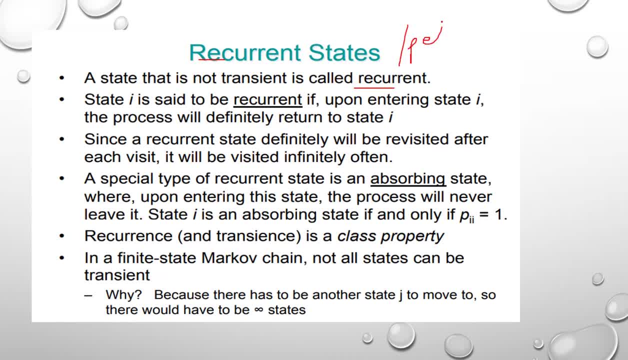 recurrent of first system. okay, see, this is also said. i said to be recurrent if, upon entering state i, the process of development definitely returns the same state i. this is the definition of the recurrent or persistent, since here is recurrent state definitely will be revisited after each. 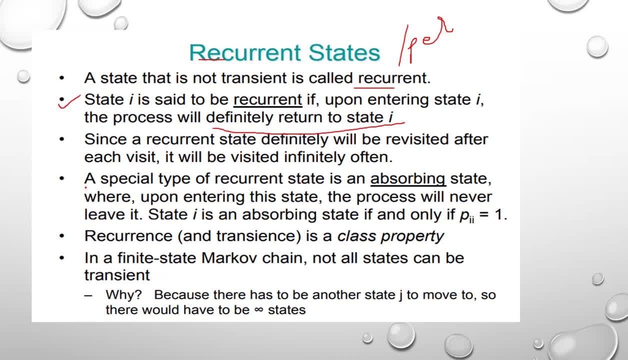 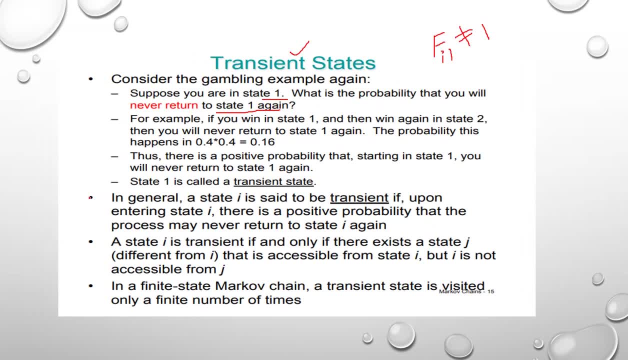 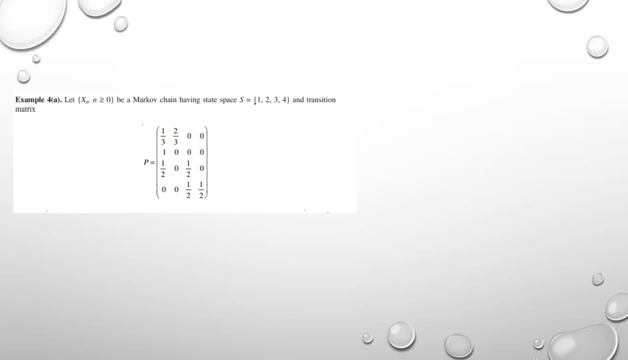 visit. it will be visited infinitely often also. these are all things also points to remember when you are doing communication, communication problems. this is also transient when you see the examples that time you can easily understand. see, this is my example. there is four classes. first formulate graph. we don't need calculation. i will tell you some. 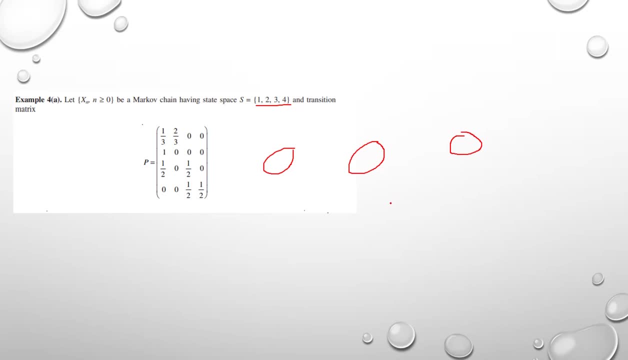 simple tips for this type of questions. we don't need calculation by just graph. we can say: if 1 2 1 is 1 by 3, 1, 2, 1 is 1 by 3. 1 2- 2 is 2 by 3. 1, 2, 2 is 2 by 3. 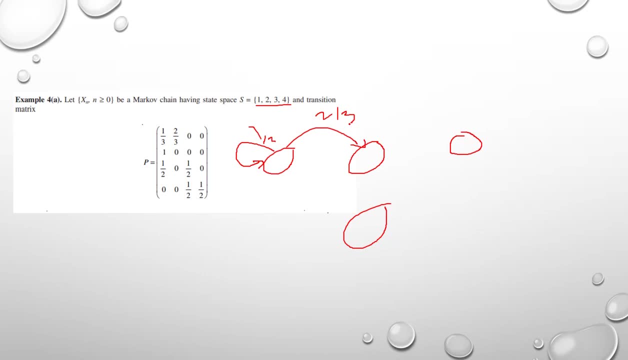 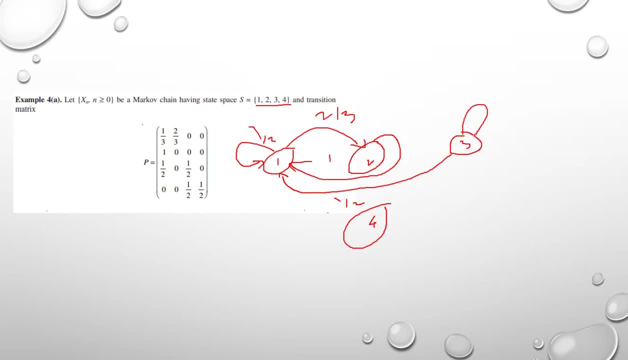 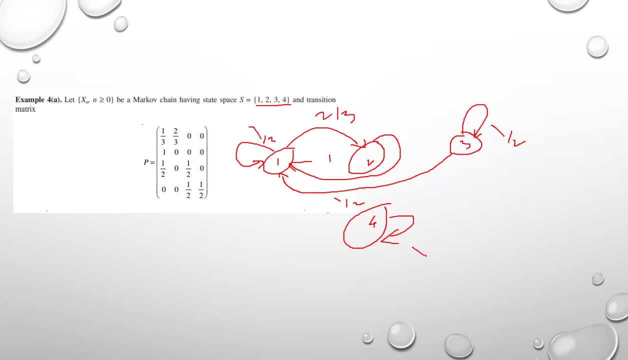 4 2. 4 is 1 by 2, 4 2. 3 is 1 by 2. this is reducible or reducible chain. this is by seeing the graph here says that it is reducible. it is reducible Chinese. 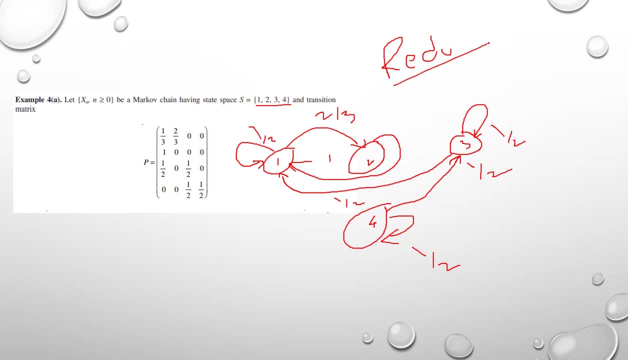 reducible chain. now we can calculate persistent and recurrent or transient state. if you observe, ok, observe class 1. ok, by observing class 1, what you understand? first, we have the same thing. and second, when going from class 1 to class 2, return also there. so it is. 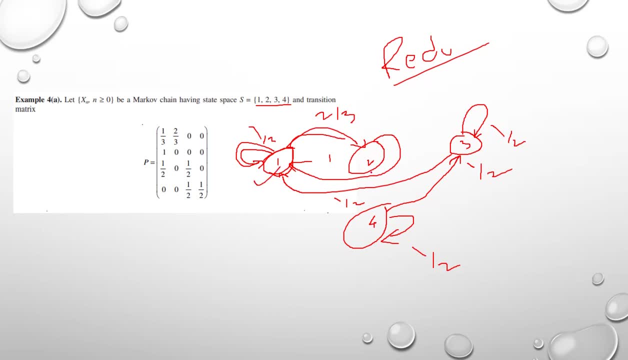 persistent. ok, for class 2, from 2 to 1 is possible. 1 to 2 is possible, so it is also persistent. when you check for 3, see 3 to 1 is going, but there is no any back step from 1 or 2 to 3, so it is. 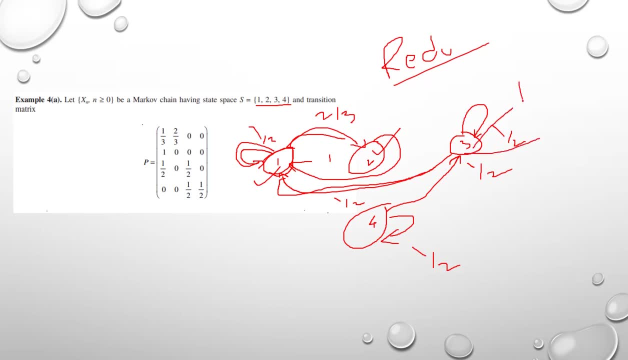 transient, is transient, transient. these two are persistent. when you take for 4, also 4 to 3 is going. there is no back from 3 to 4, so it is also transient, is also transient. this type of examples are there, we don't need calculate all. 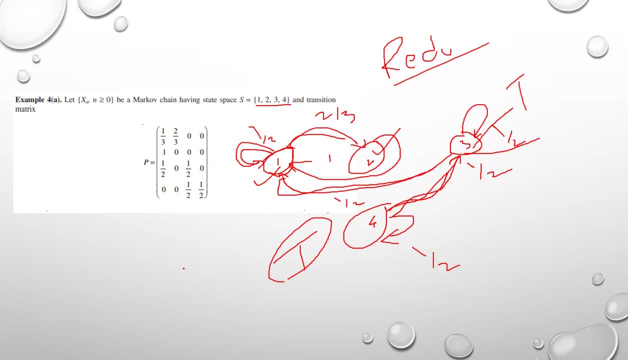 calculations. also by seeing translation transition graph you can say if classes are persistent or recurrent. then we can find mu 1, 1, mu 2, 2, also by applying formulas. ok, you can calibrate this. now we can move to the one more example. this is also important example. see now I am. 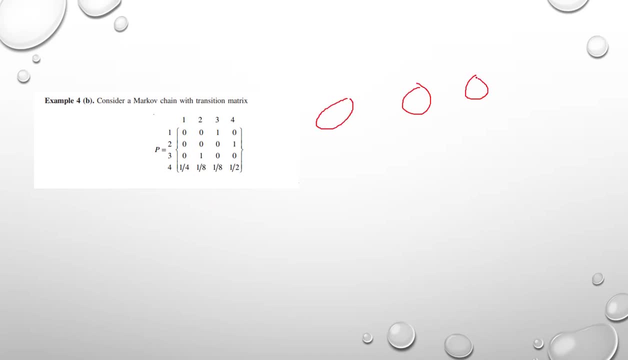 to be juxtagl empathy from respect to performance of over graduation, unless 1po to double configuration as the result. now, if you do complement for thiseded todling 16202, oh, graf is important. 124 Problem: eat one or two. this is a particular result so that any left over the contract to get. 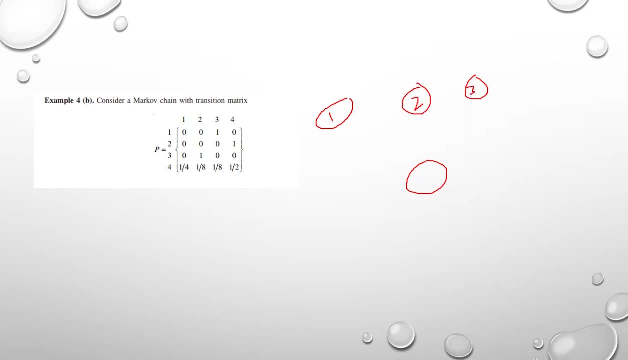 any. the contrast is not too much, and this is arazhch vocal mask: planeta moon mahnan. one dollar graph is important one, and that, in this case, the media is stored in a three, four, from three to one, two, three, sorry. one two, three is one, one, two. three is one, two. 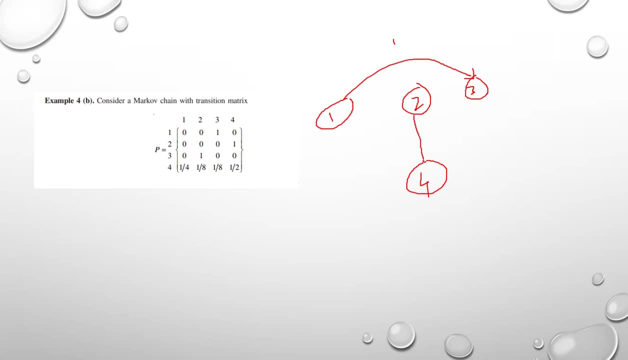 two, four. two, two, four is one, then three, two, two is one. from four to one possible, four to four possible. here everything is possible. four to one is possible. four to two possible. four to three possible. four to four is possible. now we can check. take class one for class by. 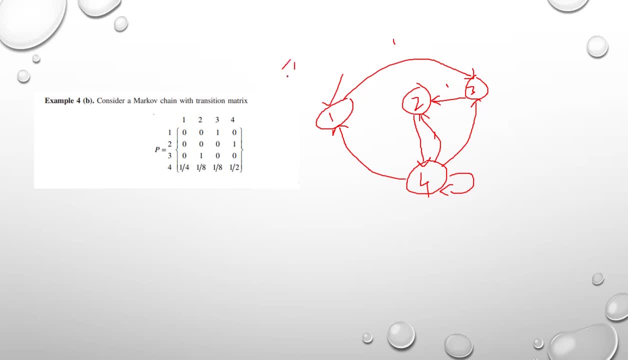 observing, it is irreducible. irreducible communication is possible for each and every class, so it is irreducible. one, two is three, going on three, two, two, two, two, four and four to one. so it is what persistent. you can take class two also. there is relationship. so 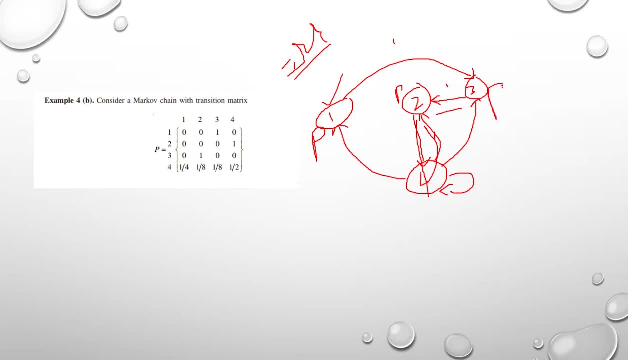 it is also persistent. you can take class three. it is also persistent. you can take class four. it is also passing. so, by using the irreducible property, if one class is persistent, then all classes are persistent. okay, this is persistent. and ergodic also. we can discuss ergodic in next videos. this: 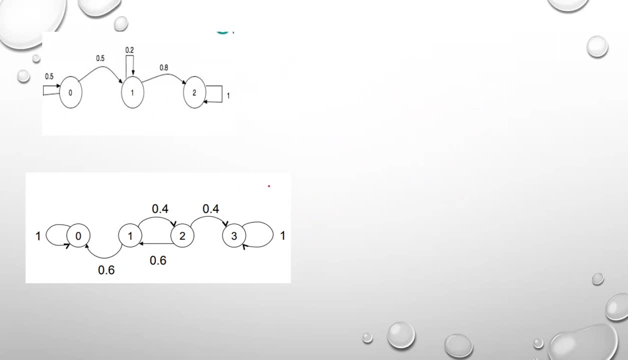 is persistent and ergodic. also, we can discuss ergodic. see this video, see this question. this is: these are these two? are class zero to one and one to two? classes are there? by observing, we says that it is reducible chain. then zero is what? zero is transient and one is also transient. 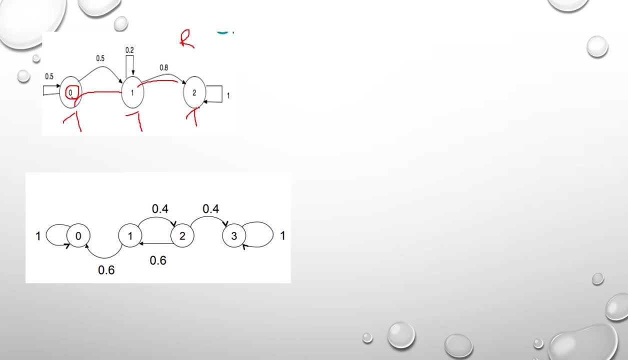 two also transient. there is no any persistent class. okay, sorry, sorry. two is persistent. two is persistent. one and two are transient because from two to one there is no any step, so two is persistent. okay, now i can move to the. this examples also say: from zero is persistent class, zero is persistent. then 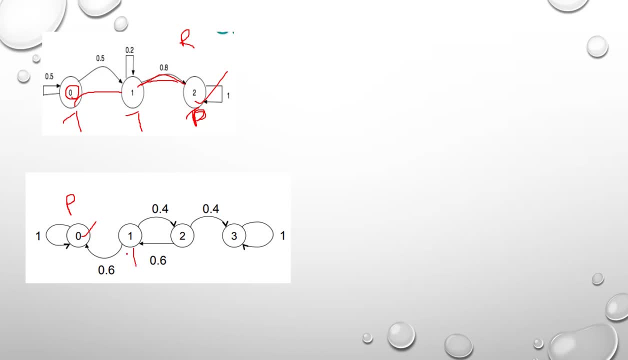 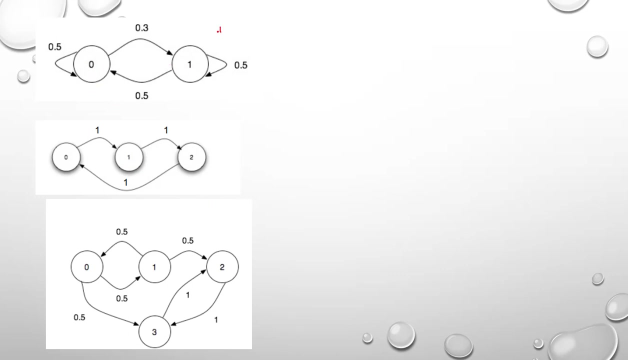 one, one is transient because from zero to one steps, not there. two, two is persistent or three is transient. okay, you can observe, you can easily understand this also. you can see these examples also. this is irreducible chain, all are persistent. by easily. you can see this communication is there. we can say that this is persistent and it is reducible.